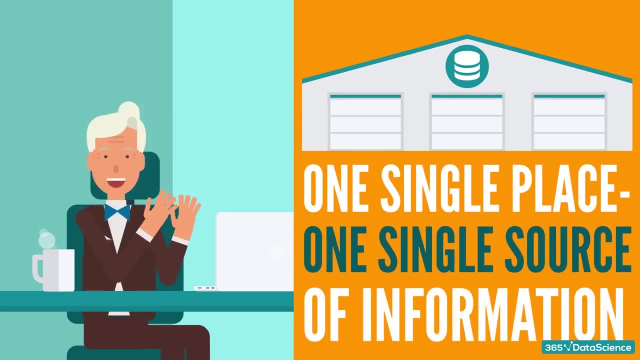 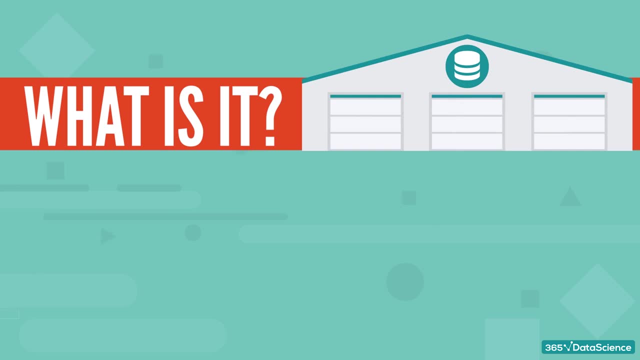 source of information. That would be quite helpful, wouldn't it? Well, a data warehouse exists to fill that need. So what is a data warehouse exactly? It is the place where companies store their valuable data assets, including customer data, sales data, employee data. 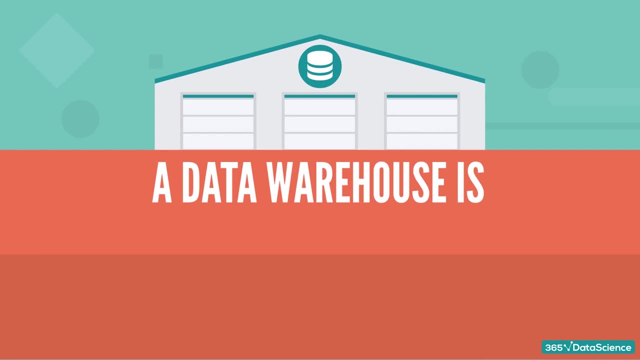 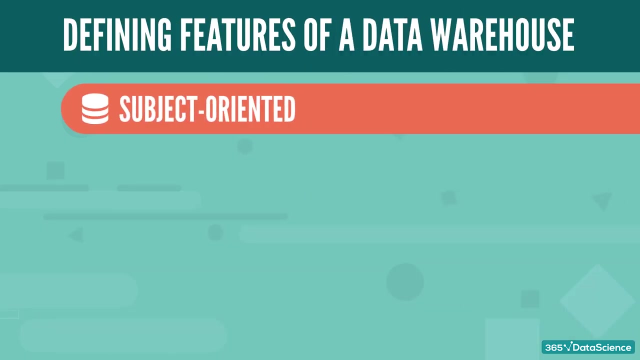 and so on. In short, a data warehouse is the de facto single source of data truth for an organization. It is usually created and used primarily for data reporting and analysis purposes. There are several defining features of a data warehouse: It is subject-oriented, integrated, time-variant, non-volatile. 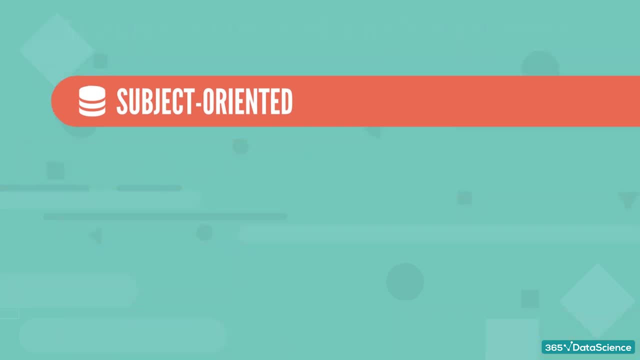 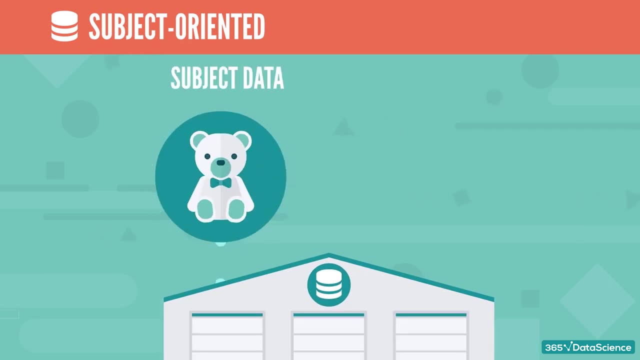 summarized. Let's quickly go through these one by one. Subject-oriented means that the information in a data warehouse revolves around some subject. Therefore, it does not contain all company data. It is not a data warehouse. It is a data warehouse. It is a data warehouse. It is a. 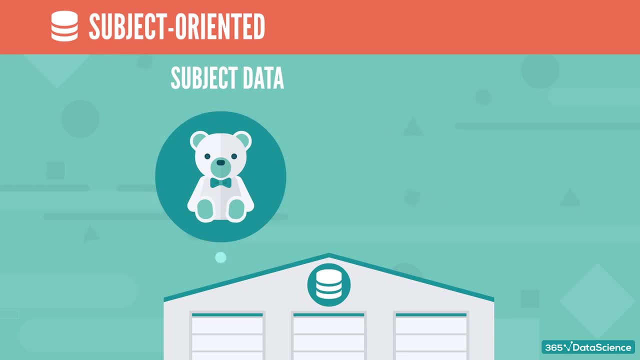 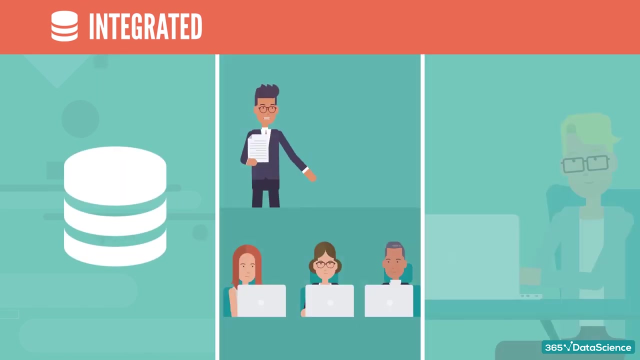 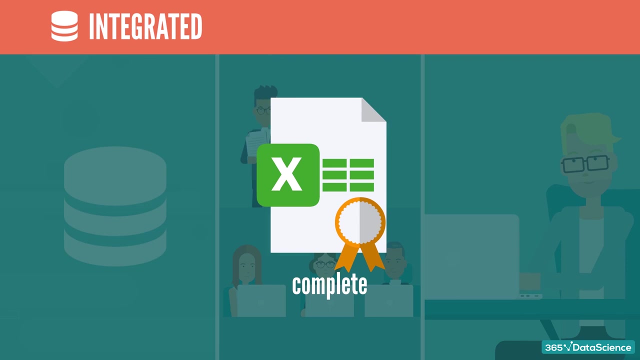 data warehouse. However, your own sales data will most certainly be there. Integrated corresponds to the example from the beginning of the video. Each database, or each team, or even each person, has their own preferences when it comes to naming conventions. That is why common standards are developed to make sure that the data 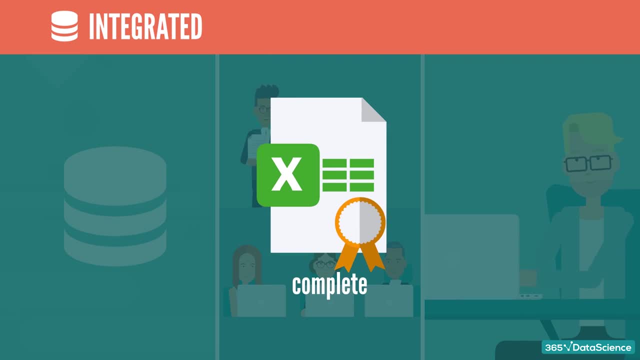 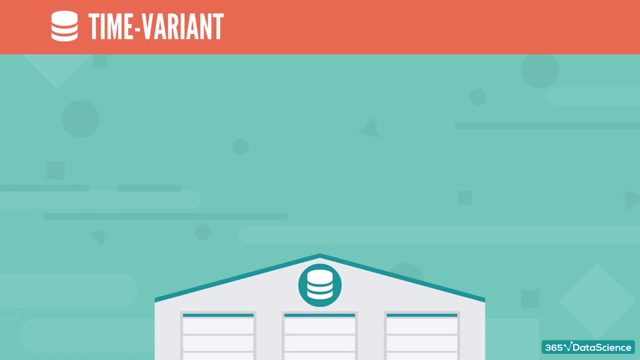 warehouse picks the best quality data from everywhere. This relates to master data governance, But that is a topic for another time. Time-variant relates to the fact that a data warehouse contains historical data too. As said before, we mainly use a data warehouse. 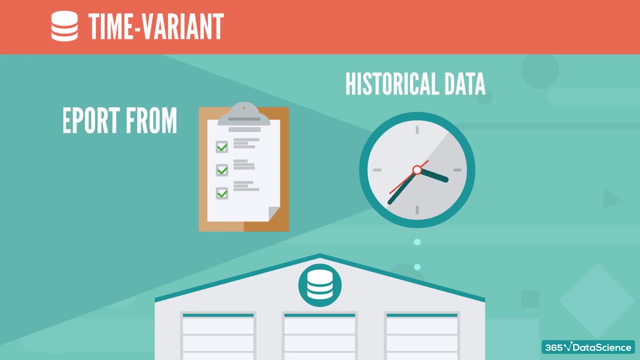 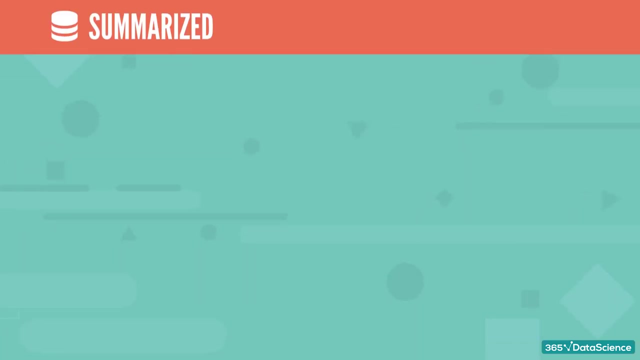 for analysis and reporting, which implies we need to know what happened 5 or 10 years ago. Non-volatile implies that the data only flows in the data warehouse as is. Once there, it cannot be changed or deleted. Summarized once again, touches upon the fact that the data is used. 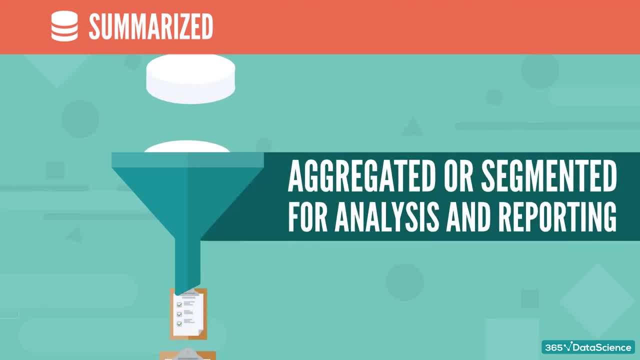 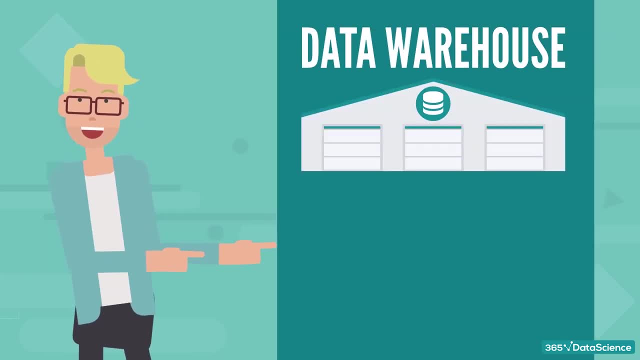 for data analytics. Often it is aggregated or segmented in some ways in order to facilitate analysis and reporting. Alright, so that's what a data warehouse is: a very well-structured and non-volatile de facto single source of truth for a company. If you enjoyed this video, 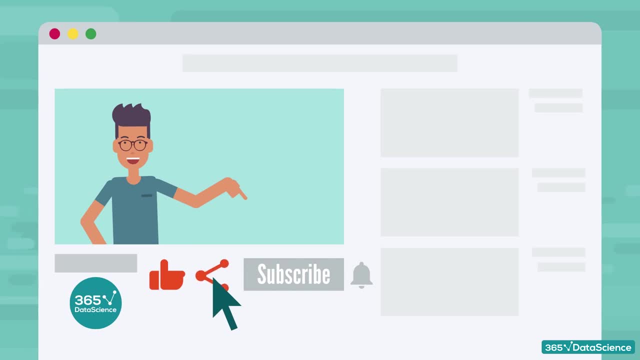 don't forget to hit the like button and share it with your friends, And if you'd like to become an expert in all things data science, subscribe to our channel. Thanks for watching and good luck. Transcription by CastingWords. 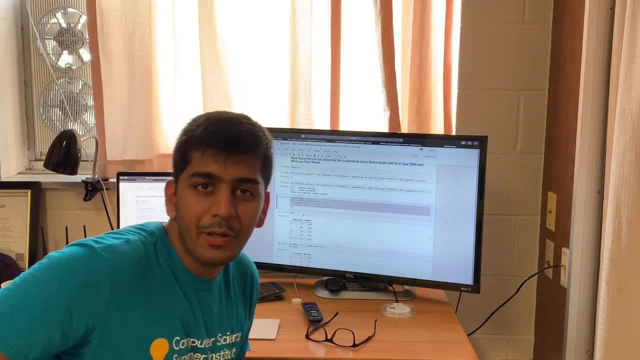 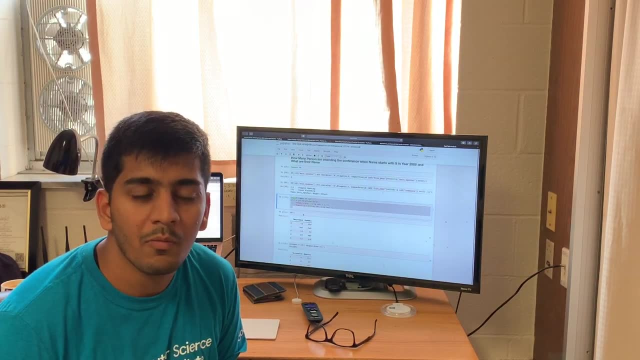 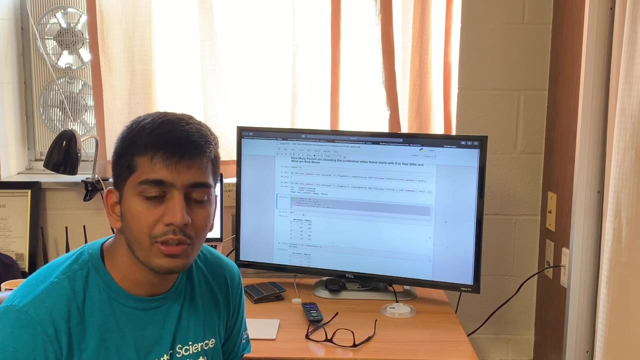 Oh, hi there. How are you guys doing? I hope you guys are doing fine. This is one of the most important topic, which is data cleaning in Python pandas. So one of the important problem when you are doing machine learning or any kind of data analysis is using is basically data cleaning. So the most important part is data cleaning. So what, what do you mean by data cleaning? Maybe you have zero values, maybe you have none values, maybe you have na, or how do you handle all all of these? So how do I fill? 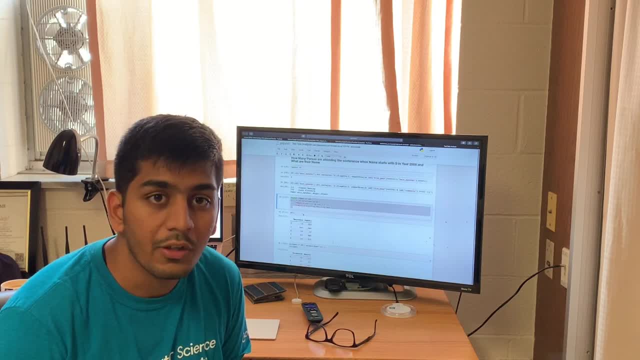 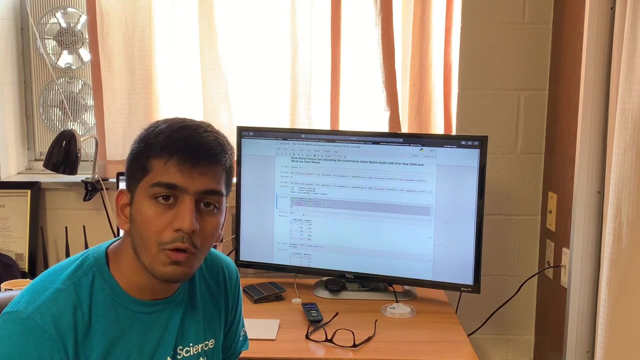 So first of all, we'll learn how to remove all these values using drop, And also we will try to detect various na values which your is null- won't detect. So we will learn all of that. Once we will learn all of that, then after that we will see f fill, b fill, So forward, fill, back fill. then we're going to learn interpolation- How do we manipulate data. So we will learn all of that in this tutorial of data cleaning with Python and pandas. So if you have any questions, 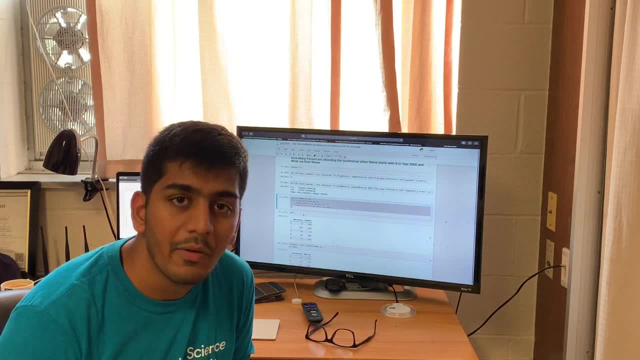 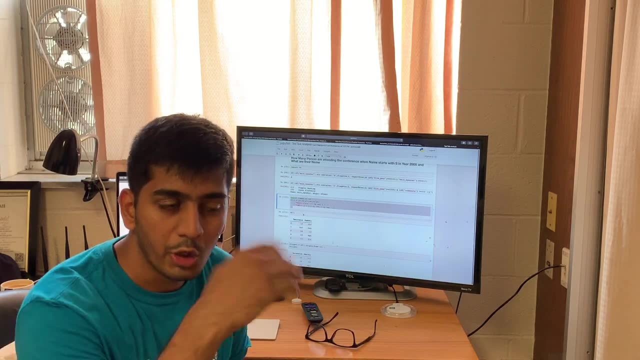 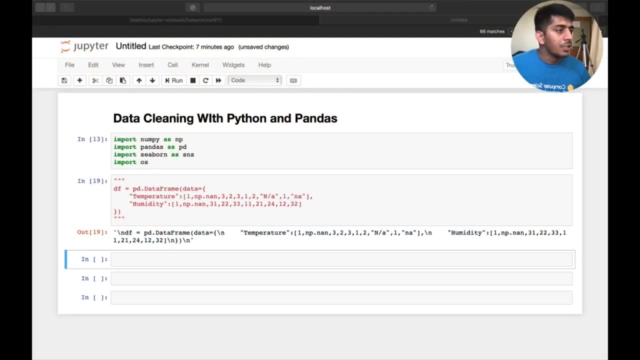 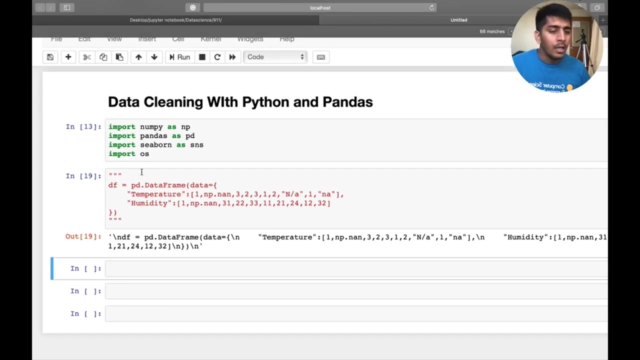 make sure to post your question in the comments And I will be very happy to answer all of your questions. So let's not waste time and get back straight into coding. So join with me on the tutorial series right now. Welcome everyone to the video series. And in this video we will learn the art of data cleaning with Python and pandas. So we will use a lot of methods to visualize the data, the data that is null data. we will try to fill the data using backfill, forward fill b fill, and then we will learn how to do that. So let's get started. 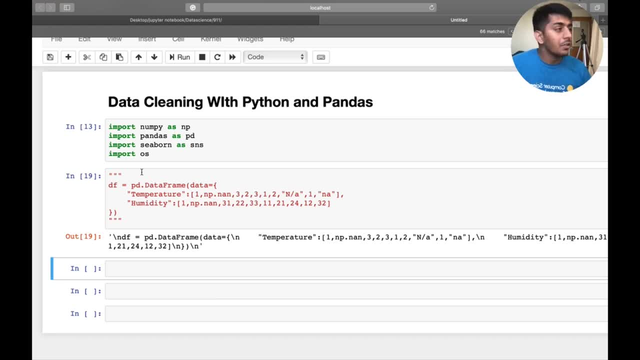 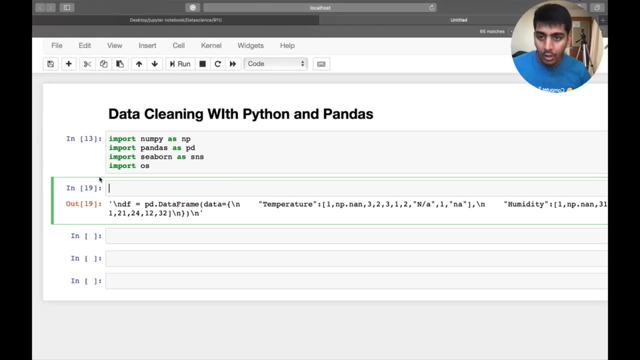 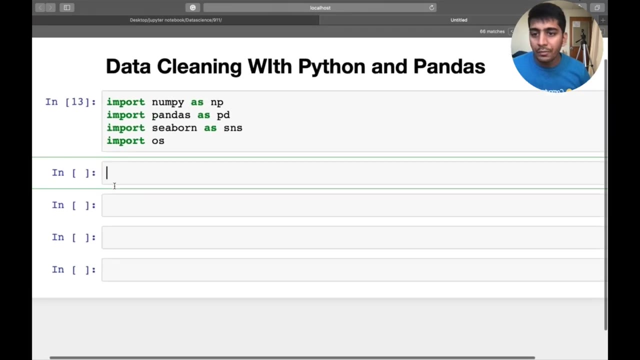 interactive. So now let's see. So first of all we need NumPy, Pandas, Seaborn and the OS library. So first of all, I'm just going to make sure that the file is already there. So I'm going to say list dugs And I'm going to paste it into M定s And I'm going to uncompress it and paste it in the intox ether. So once again,